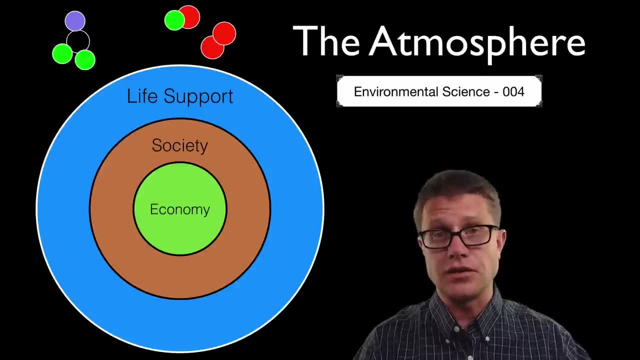 how do we solve that problem? Industry is going to say, rightly so, we should not have to bear the cost of all of this. It is going to cost us millions, if not billions of dollars. We are going to lose jobs. But eventually the consensus came around and government said: 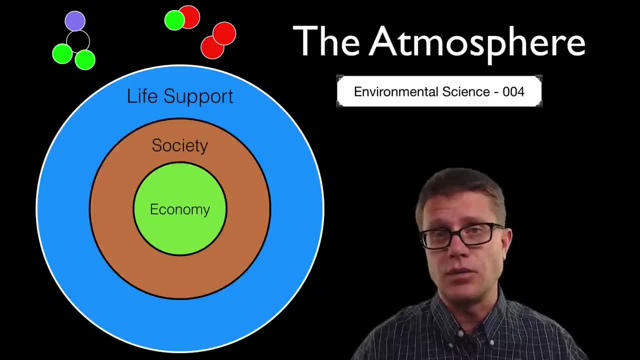 we are going to have to solve this problem. And in 1987 they signed on to what is called the Montreal Protocol, where they banned CFCs. That has led to a decrease in CFCs. increase now of ozone. It will increase in CO2.. It will increase in carbon dioxide. It will increase. 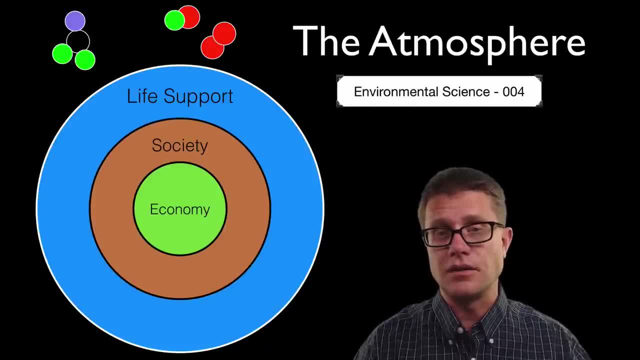 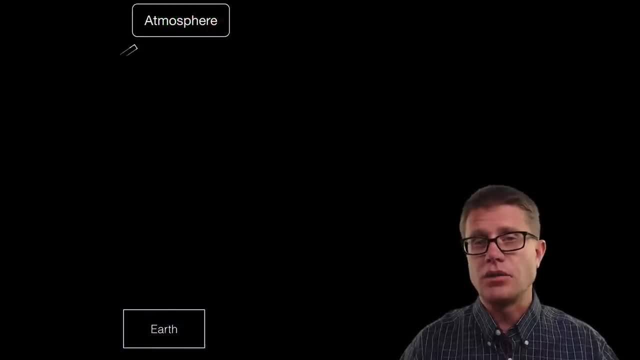 in oxygen. It will probably return to its original levels by 2050. And so this is a great example of how governments can bind together to form a treaty that is incredibly successful. And so the atmosphere surrounds the earth. Scientists break it into a number. 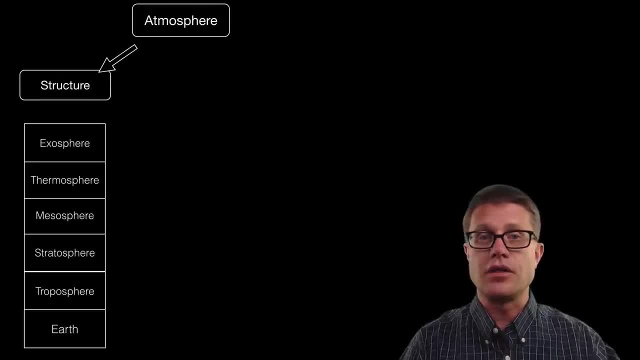 of different spheres. We have got the tropostrato, meso, thermo and exosphere. Now we live in the troposphere and that protective ozone is going to be found right at this boundary between the two. Weather is going to be the current state of our atmosphere And over. 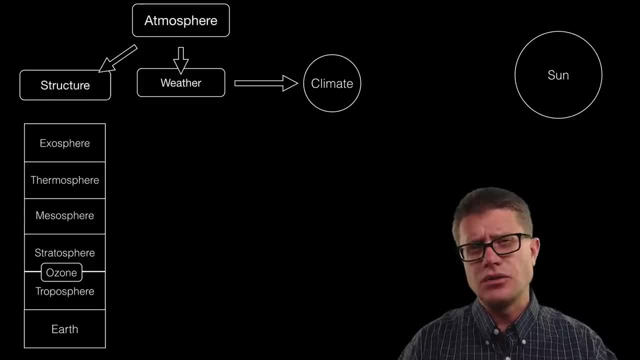 a long period of time. we call that climate, Which is due to the tilt of our axis and where we are in the orbit around the sun, And so, due to our location, we get seasons: We are pointed towards the sun in the summer and away from the sun in the winter, But also 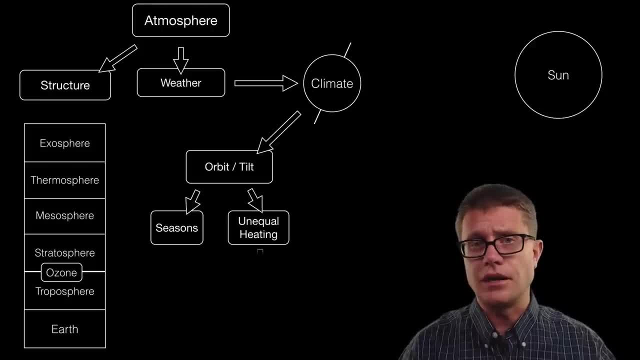 since we are a sphere, we are starting to get unequal heating of the planet, And those convection currents lead to cells in the atmosphere. We have got things like the Hadley cell, the Farrell cell, And what those are doing is moving the atmosphere around on our planet. 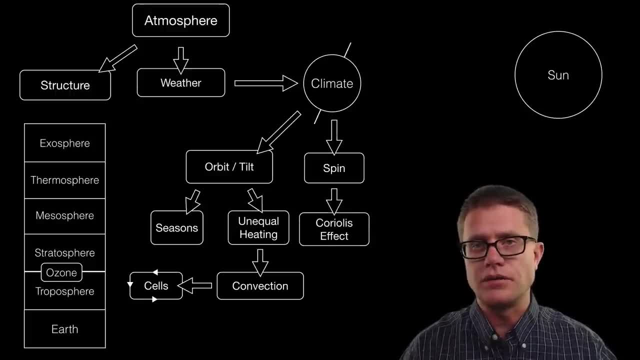 Now we also have a spinning planet, And we have a spinning planet And we have a spinning planet, And that creates something called the Coriolis effect, And so it spins in a characteristic way, And so the combination of these two lead to atmospheric circulation. 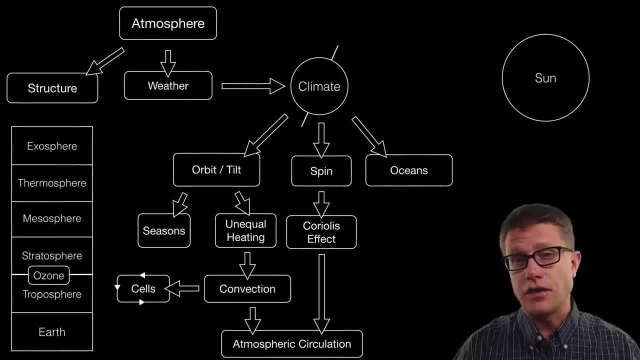 It is moving the weather around on our planet. Now the oceans also affect our climate, And as the atmosphere moves around, it starts to move the oceans, And so we get these ocean currents which are shaping our climate, And an example of all these things coming together. 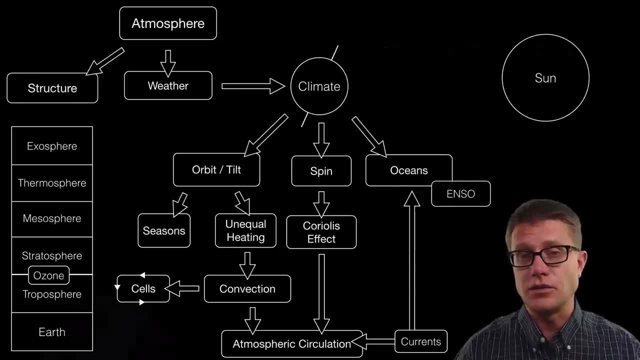 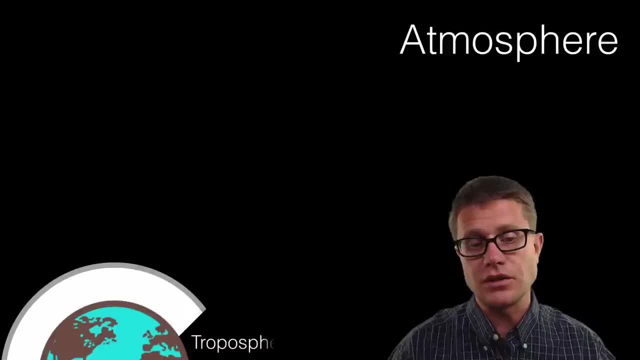 is El Niño, or Enso The El Niño- Southern Oscillation, which we will talk about in a little bit, And so the atmosphere is a series of currents that are moving around on our planet. This is not to scale, But the lowest one is going to be the troposphere. That 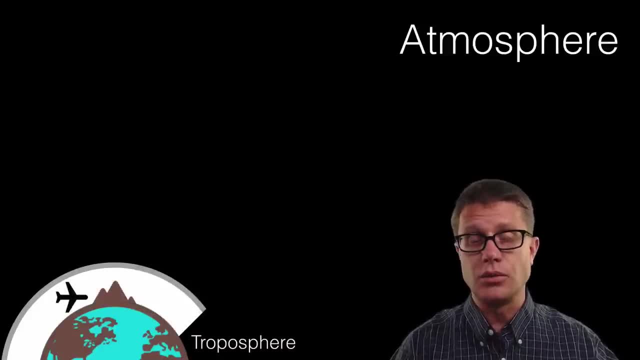 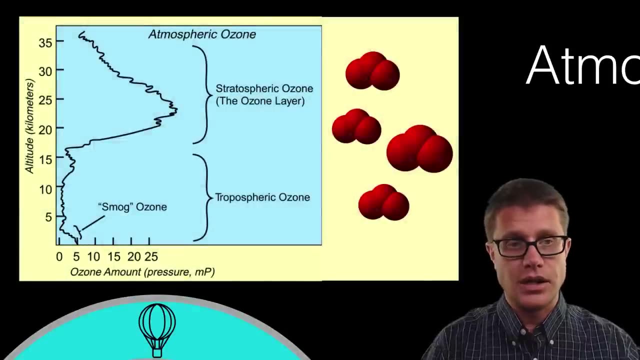 is where our mountains are. That is where we are. When you are on a jet, you are still within the troposphere. Above that we are going to have the stratosphere, So weather balloons will move into that area If we look at ozone right here. So this is going to be. 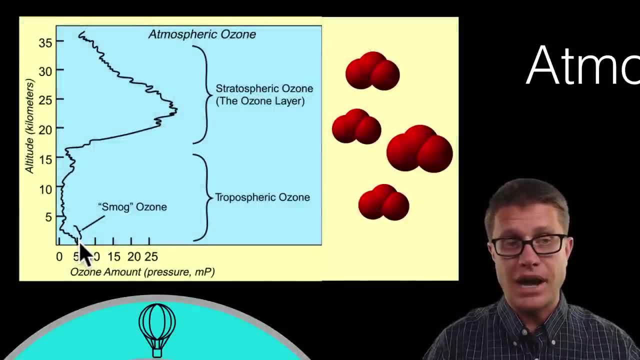 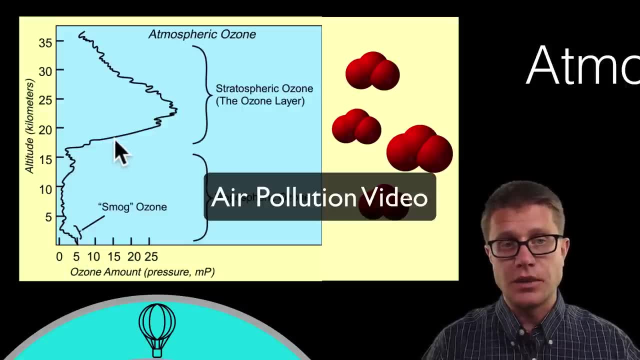 ozone. right at the surface of the planet We are going to have some bad ozone. We call that tropospheric or smog ozone. that can be damaging to us. We will talk about that later. But as we move up in the troposphere into the stratosphere we are going to have a huge 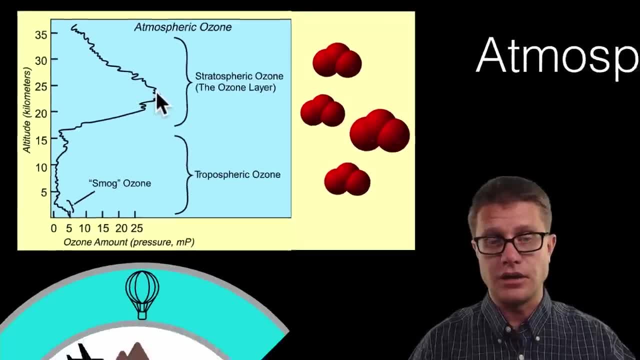 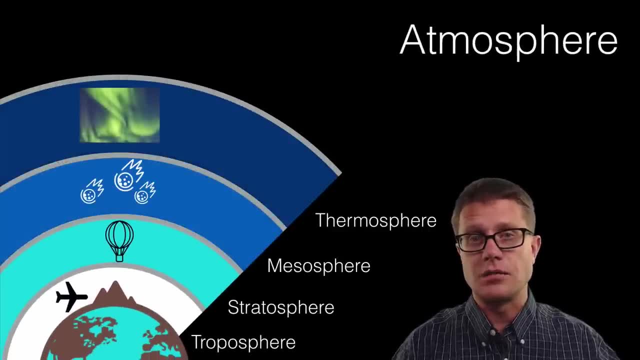 increase in that ozone layer, That is that protective layer around us. Above the stratosphere we have the mesosphere, That is where meteors are burning up. Above that we have where the aurora are. That is going to be the thermosphere And then, finally, we are bordering space. This 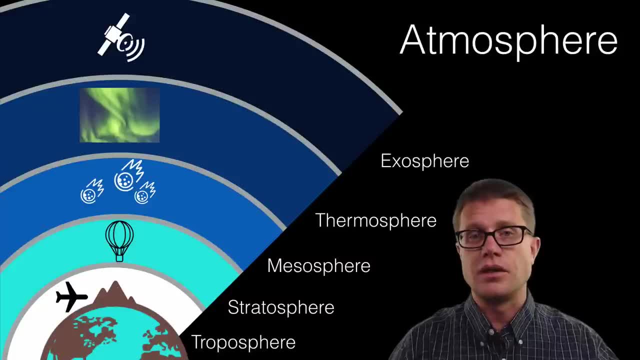 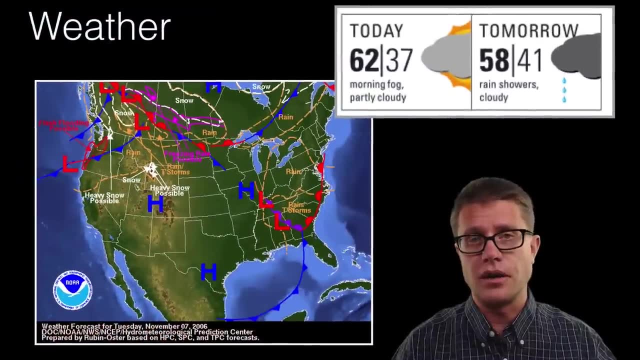 is going to be the exosphere up here Now. what are some conditions within the whole atmosphere? We are going to increase density the closer we get to the earth, because there is higher gravitational pull, the closer we are. Now what is the atmosphere like today? 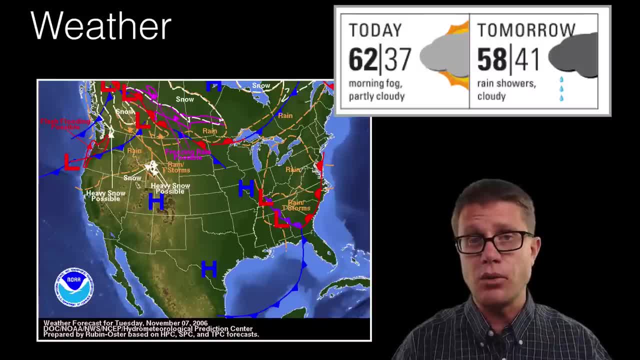 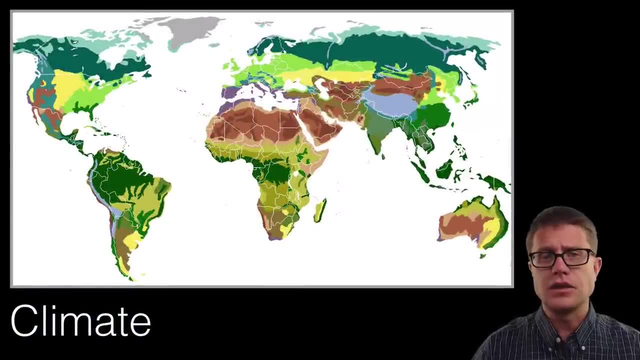 That is weather. Is it raining, Is it sunny? What is the temperature? And that is important. But what is more important is climate. That is going to be weather over a long period of time, And if we look at this biomat, you start to see some patterns. And so if you 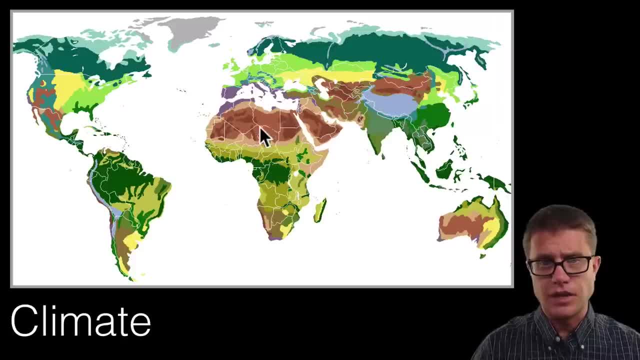 look, right here we are going to have a bunch of tropical rainforests, We will have deserts right here. And if I put the latitudes over this, the one thing I am always surprised is how low the equator is. So if we put this in at 0 degrees, then 30 and then 60, real 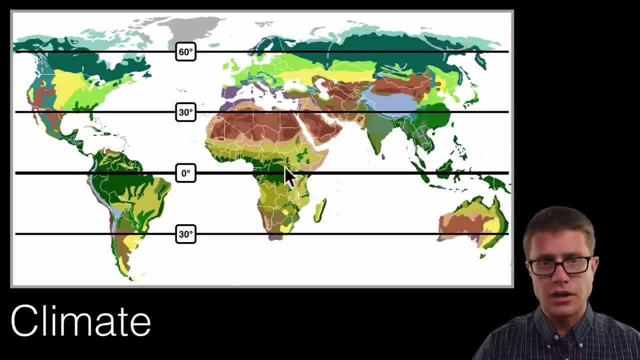 patterns start to emerge. So right here along the equator, we are going to have all of this precipitation. Rainforests are going to start to emerge. We are going to have all of this precipitation going to be found there. But look right here, at 30 degrees above and below. 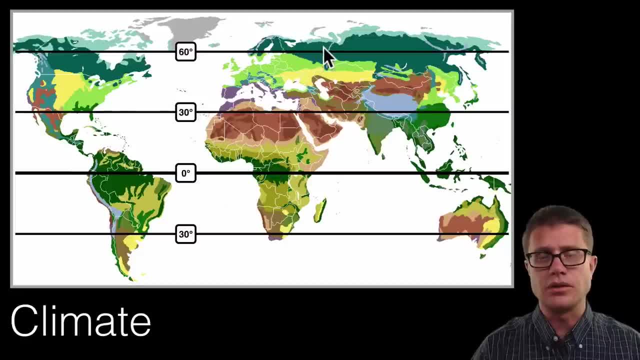 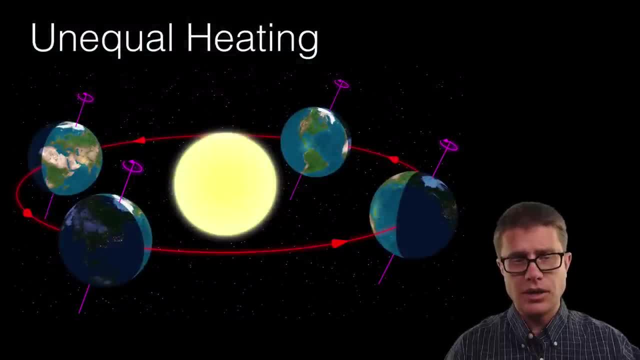 or northern and southern, we are going to have these deserts And then we are going to have these big boreal forests out here, And so all of that has to do with where the earth is in orbit and also the tilt of the earth, And so we get seasons due to the tilt. 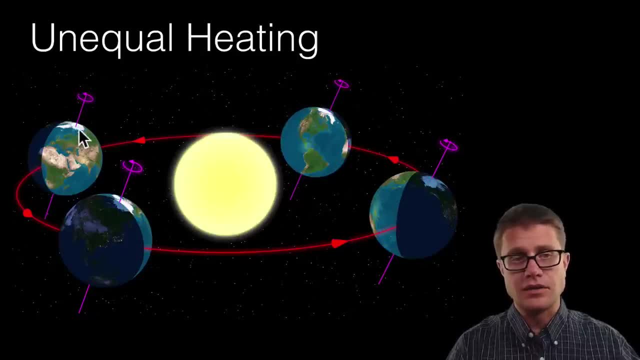 of the earth as it moves around the sun. This is obviously not to scale, But as the northern hemisphere is pointed towards the sun, look, here on the north pole it is going to be 24 hours of daylight In the winter, it is going to be 24 hours of night. 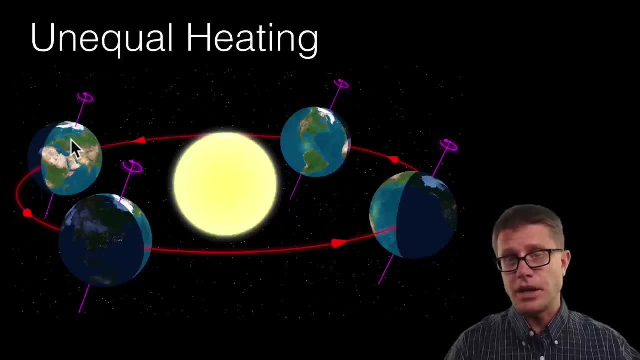 Right here we would have the equinoxes. But depending on, are we pointed towards the sun summer, or away from the sun winter, it is going to affect our weather and therefore our climate. Remember, everything would be reversed if we were in the southern hemisphere. 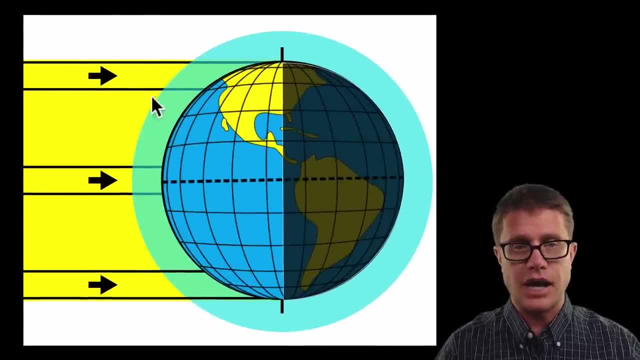 We also get unequal heating. So if I again- not to scale, but if I were to put an atmosphere in here as the sun's rays come in here at this part it is going through a very small amount of the atmosphere, So we do not lose much heat, But up here we are going through. 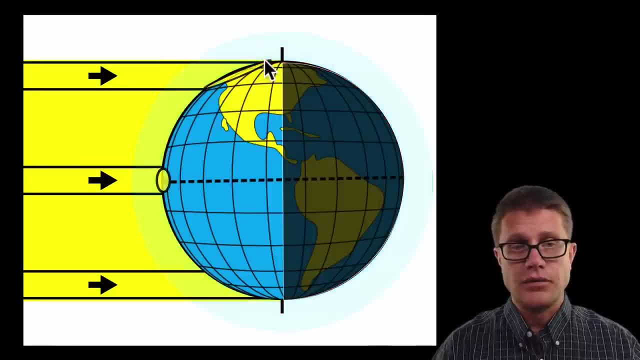 more of the atmosphere. It is going to be colder near the top If we remove that and just look at the light itself right here. this amount of sun rays is all concentrated on this very small surface area, But up here near the north pole it is. 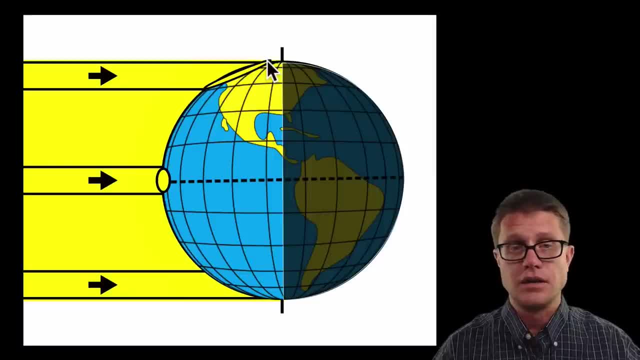 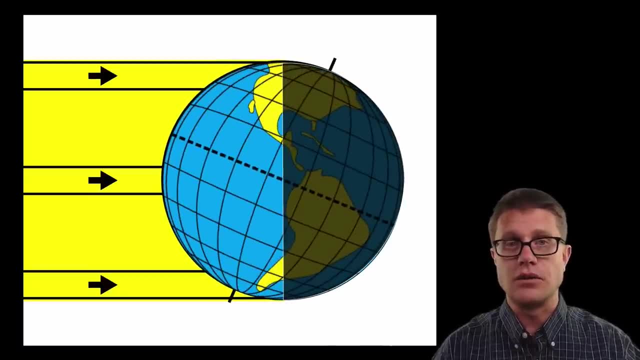 spread out over a long surface area, a large surface area, So it is going to be cooler near the poles. Now, remember, as we move around, the sun that axis is going to tilt back and forth, And so that is going to affect this unequal heating And the last thing that affects 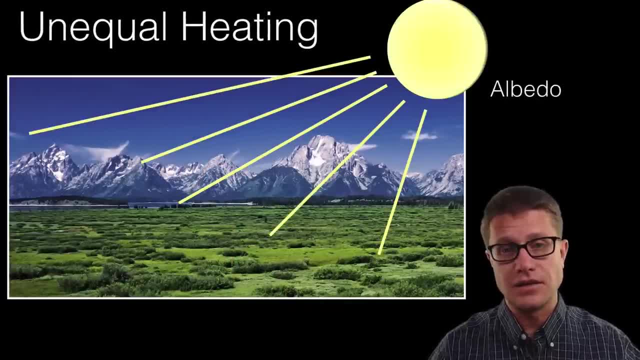 unequal. heating is the albedo of the earth. It is our reflectiveness. So as the sunlight hits the snow, for example, it is going to be reflected off, But if it hits vegetation or water, for example, we are going to have a different amount of albedo. So it is a combination. 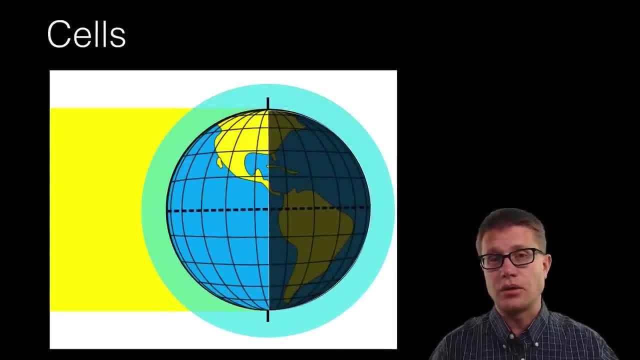 of all of these things that creates climate, The first one that is most important, are going to be the cells on our planet. What that means is, right here at the equator, we are heating up the air most right here along this point, And so what we get are these convection cells. 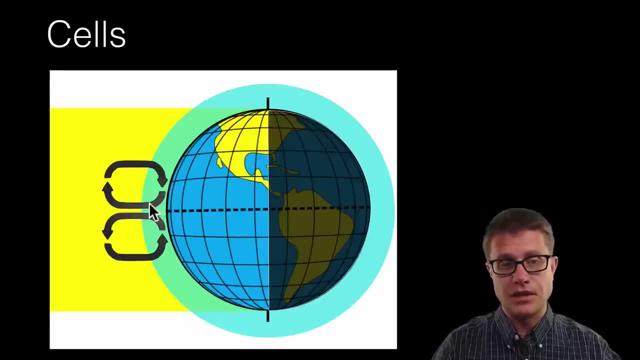 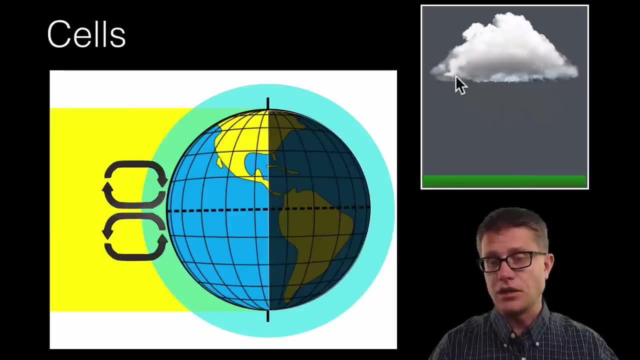 So we heat up the air and it is moving up. It becomes less dense, and it is moving up. Now, what quickly happens to it is it actually cools down. And so, as it cools down, we eventually reach something called the dew point, That 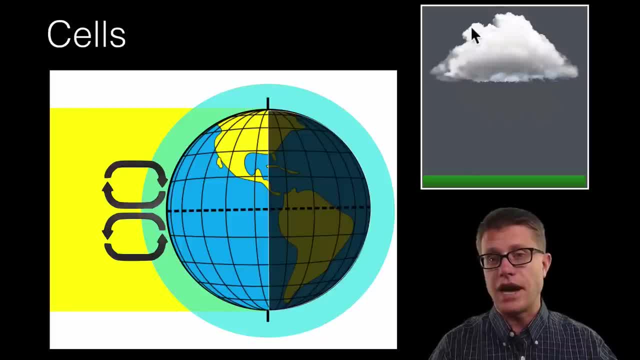 is where it cannot hold water anymore and we are going to have the formation of clouds and then we are going to have precipitation. Have you ever wondered why the bottoms of all the clouds line up? It is because we are cooling the air as it moves up until we hit. 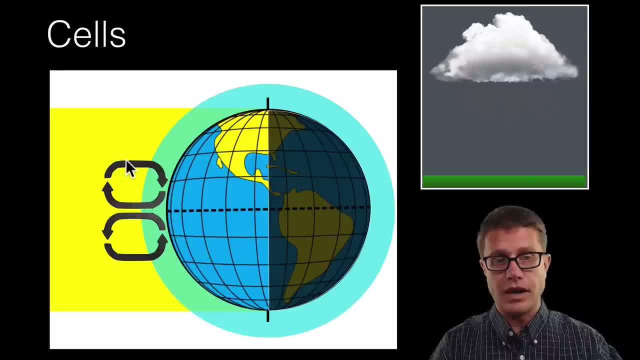 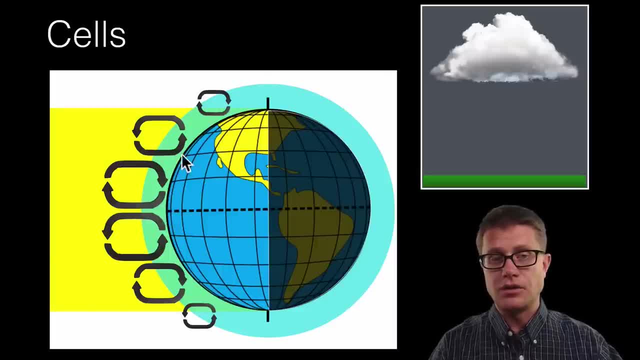 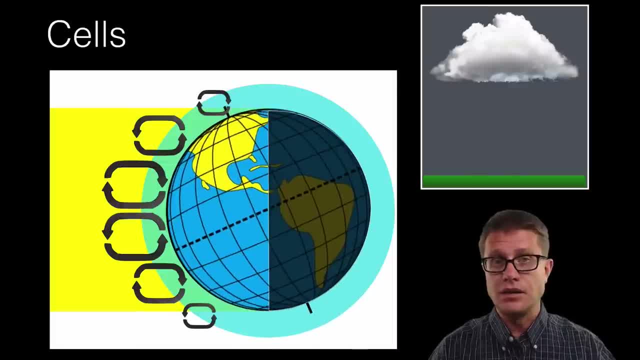 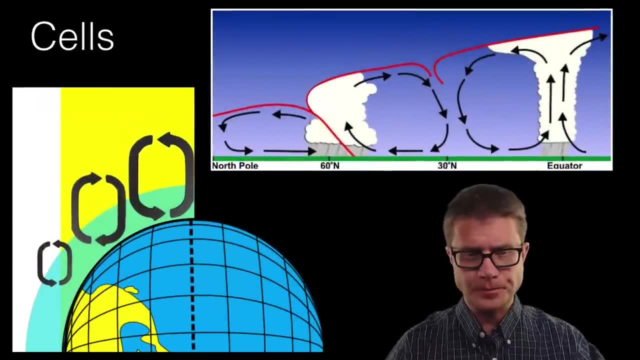 there or at the pole itself, And so these will be affected by the tilt of the earth as well, And so cells are important to understand. So I have turned the earth on its side. So this is now equator- north pole. So if we move from the equator to the north pole, the first 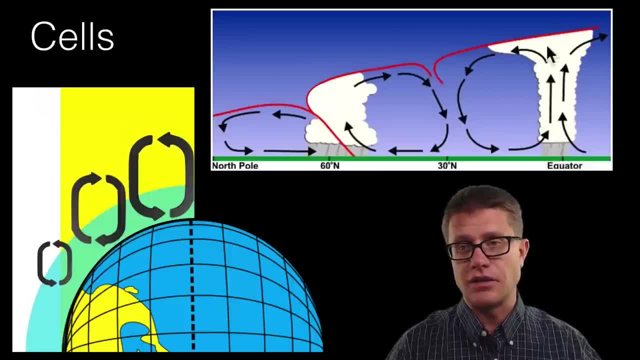 thing we see is a huge amount of convection near the equator and you are going to have a huge amount of weather. So we are going to have a huge amount of weather And so we are going to have a huge amount of weather right here. It will eventually move up and 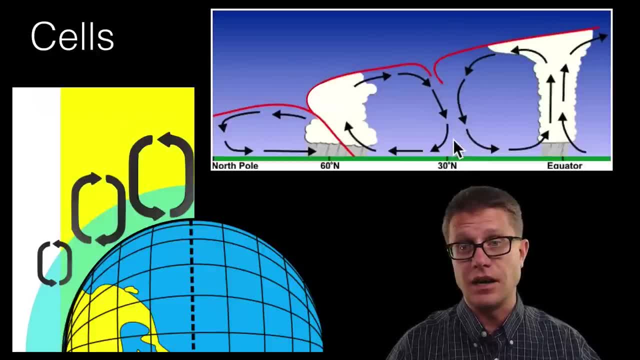 then it slides down. As it moves down, it is going to actually heat up and we are not going to have much precipitation at 30 degrees. We call this first one the Hadley cell. It is named in honor of the person who proposed it. Now, if we keep moving, so again we are. 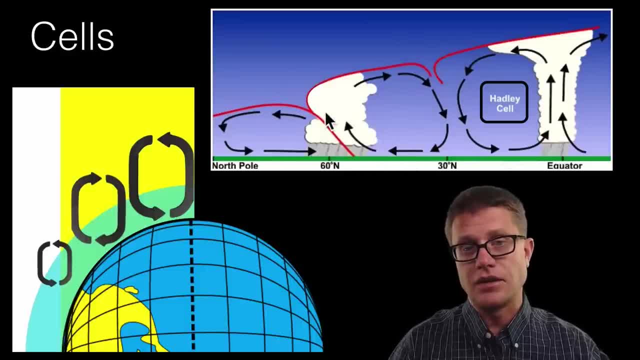 moving down to this next cell right here, we are also going to have convection current, that is moving the air up at 60 degrees north latitude and south, And then eventually it is going to be heated as it moves down, So we are going to have more precipitation here. 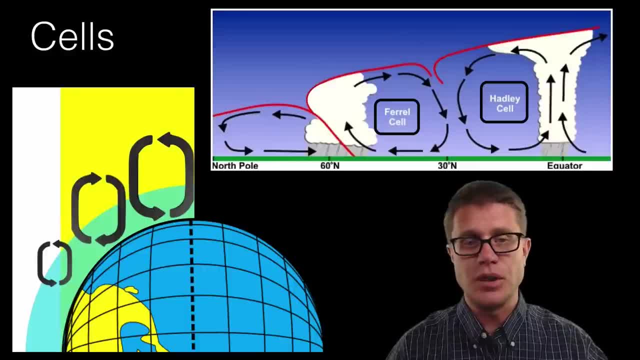 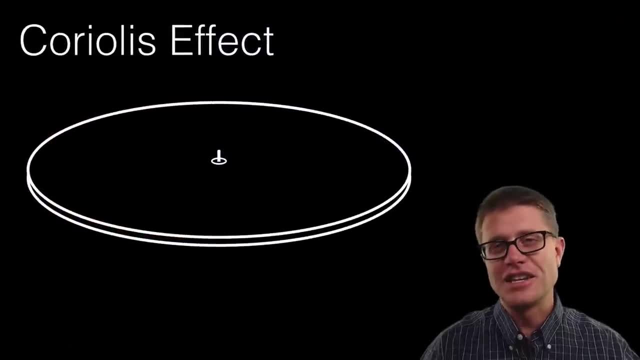 We call this the Farrell cell. It is named in honor of the person who proposed it. And then, finally, we have a polar cell. It is named in honor of- no, it is not. it is just near the pole. And so the other thing that contributes to atmospheric circulation is Coriolis effect. 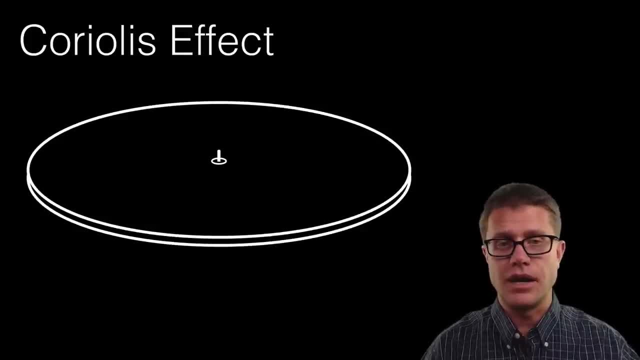 So again, the earth is spinning. Think of it like a record player spinning around. If I were to tape something to the record player, like this cone, let's say it represents the mountains. as the record player spins, the mountains are just going to move around with. 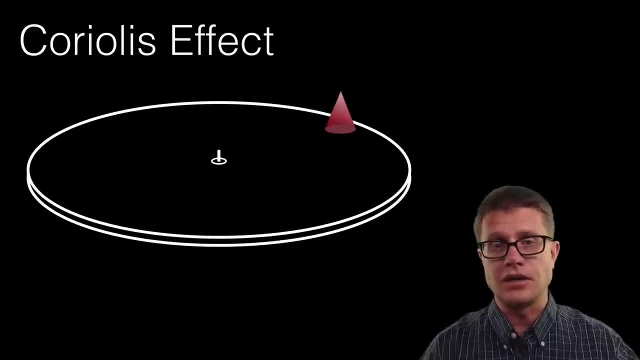 the earth. We are moving on the earth right now. We are not affected by it because we are connected to the earth. But let's say I put something on that record player that is movable. Let's say I put a marble on it And now I spin it. Watch what happens to the. 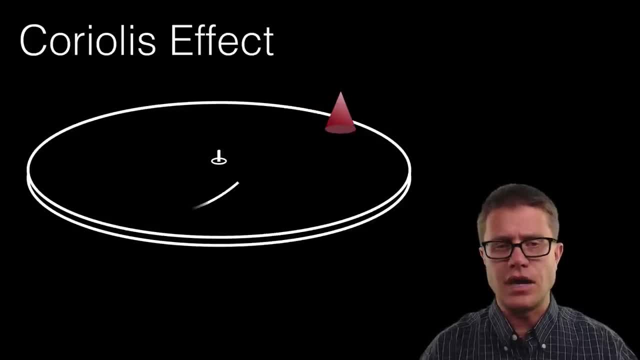 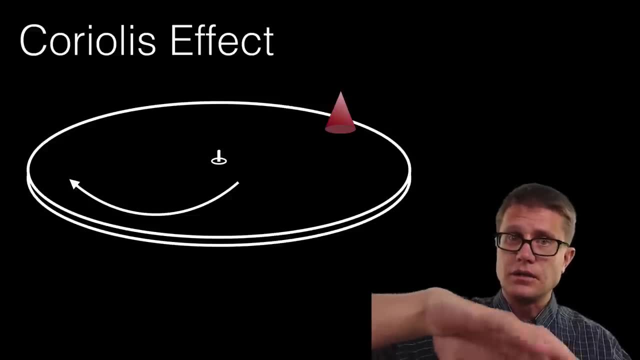 marble, It will be deflected off. And if I were to trace that path, it moves like this: And so if you think about it on the north side of the record, it is going to be moving clockwise. But if you could move underneath the record it would actually be moving counter. 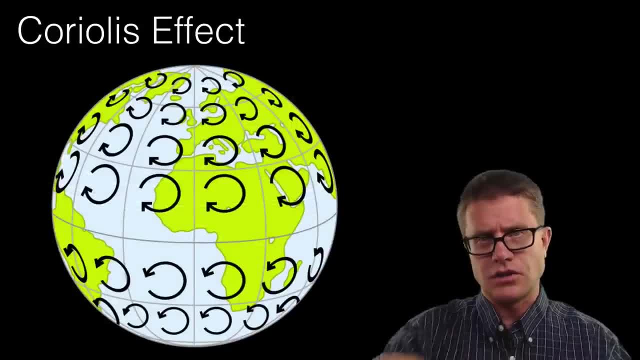 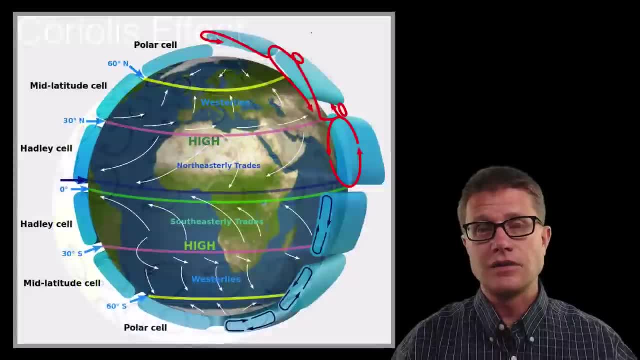 clockwise, And so the earth is like that record player. It is a sphere, obviously, but in the southern hemisphere it is going to move counter clockwise, And so the combination of these cells and the Coriolis effect creates the weather patterns that we have on our planet. 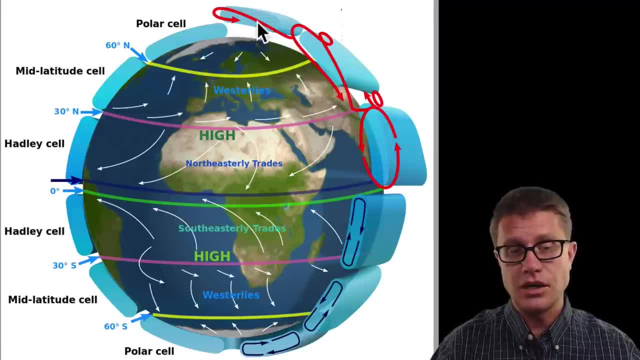 So you can see, here are the three cells- Hadley, Farrell and polar cells right here. But we also have the movement due to the spin of the earth, And so right here near the equator, we are going to have what are called the trade winds. They are always going to be moving in. 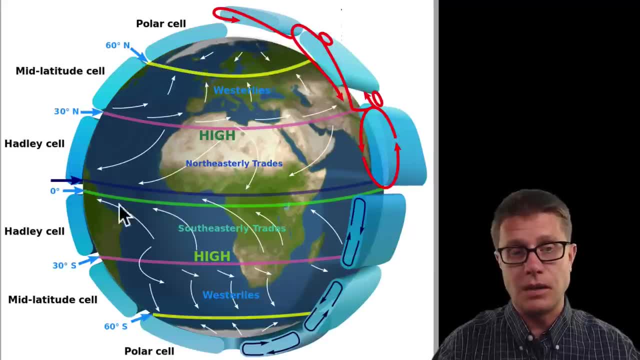 this direction due to the spin of the earth, Both in the southern and northern hemisphere. they are all moving in this direction. If we move north or south, we are going to have to start to get what are called the westerlies. It is going to be moving in this direction. 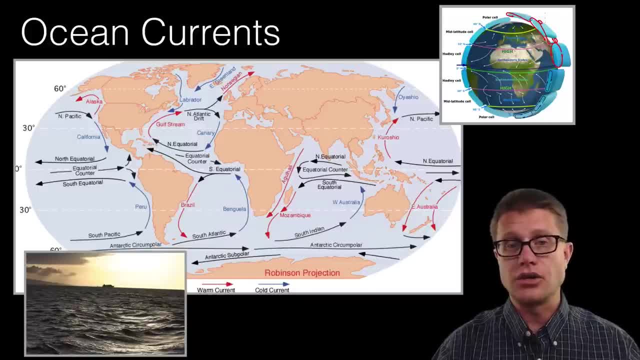 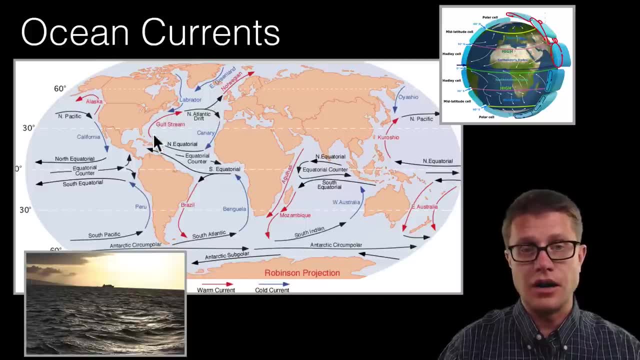 Now, as that atmosphere pushes on the ocean, we get oceanic currents, We are getting these trade winds And then we are getting the westerlies coming back. As that blows on the ocean, we get this gulf stream that is moving the ocean. We also start to get deep currents in the 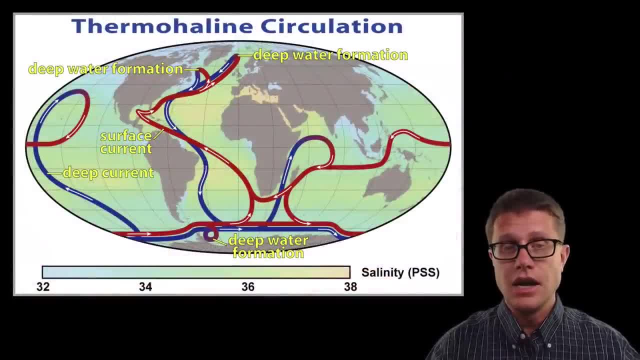 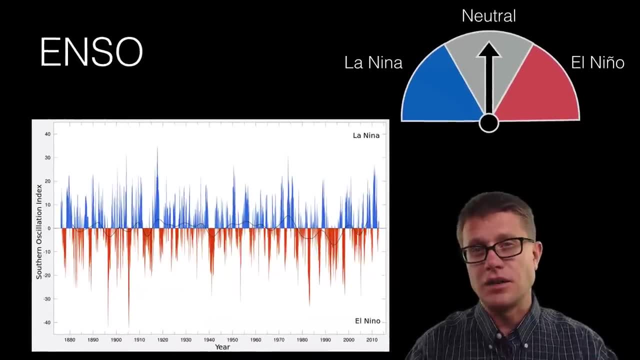 ocean due to heat, but also due to changes in salinity, And so this ocean is moving around as a consequence of not only salt but also the temperature, And so tying these all together- something you should be very familiar with- is ENSO, or. 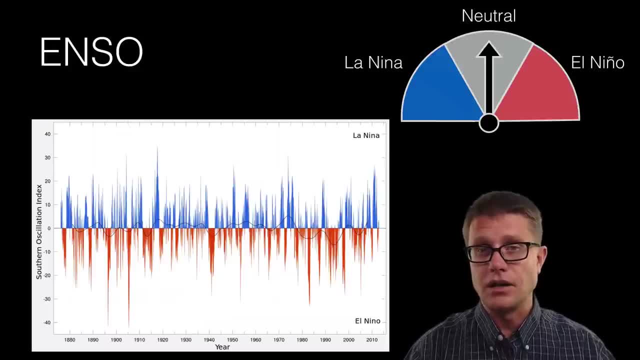 the El Niño Southern Oscillation, And what really is going on is it is just moving back and forth between El Niño and La Niña, And so this is a graph that shows this oscillation from 1880 to 2010.. And so it is in a neutral position. It will then move towards El Niño. 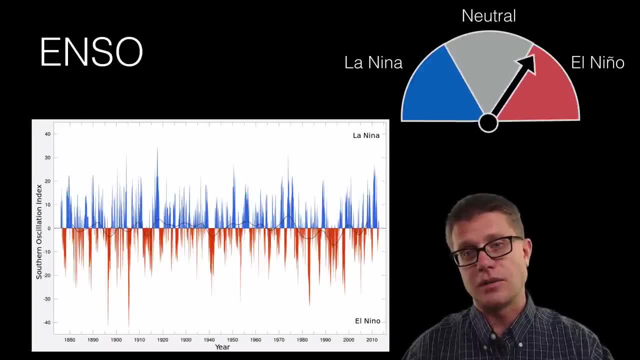 And then it will move back to La Niña, And then it will move to El Niño. Sometimes it is not a very big El Niño, Sometimes it is a very big El Niño or La Niña. It just moves back and forth, So it is oscillating. You can see that in the record, But you should. 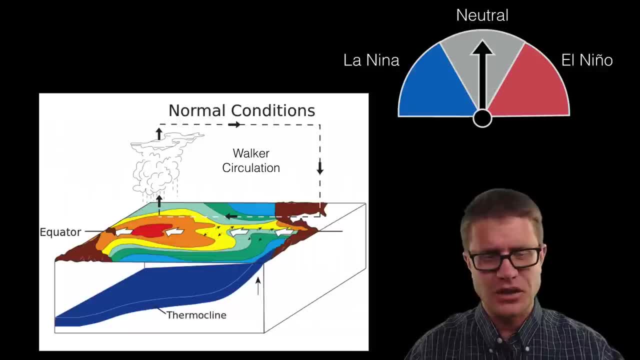 be asking yourself what causes it, And so let's go look. And so here we are looking at is the Pacific Ocean. So this is the Pacific Ocean right here. This would be Central America, South America, North America And then all the way on the other side of the Pacific is. 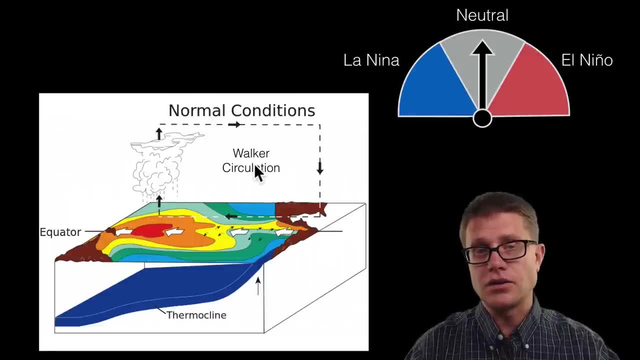 going to be Australia over here, And so what we have is a Walker circulation. Remember, the trade winds are blowing the wind in this direction, along the equator, And as they do that, what we get is a circulation pattern that moves the ocean. water, cold water here. 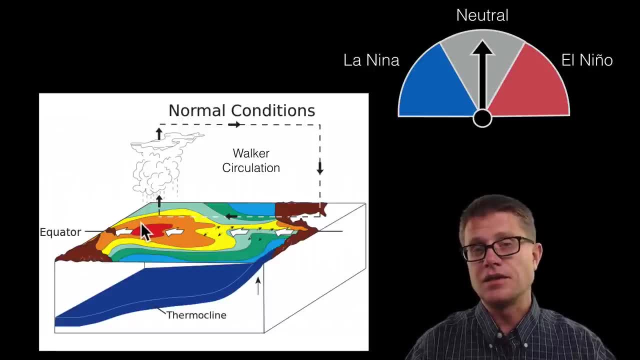 It is pushing the warm water to the Western Pacific. This is the neutral or the normal position. Now what can happen? Watch what happens to the Walker circulation as I move us into a La Niña. So, as I move us into La Niña, watch what happens to the Walker circulation.